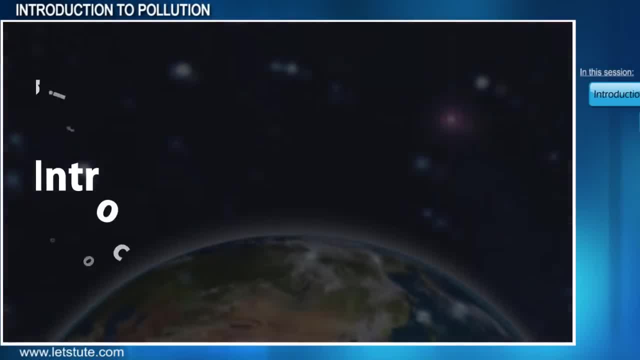 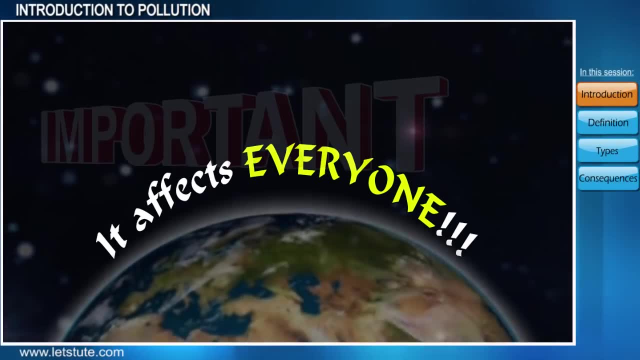 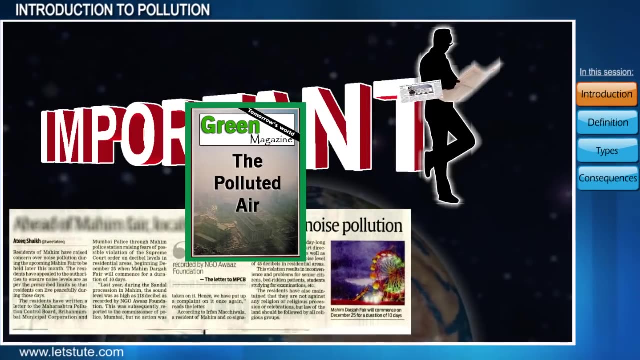 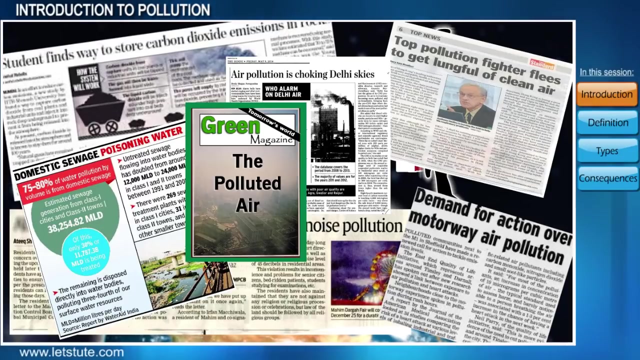 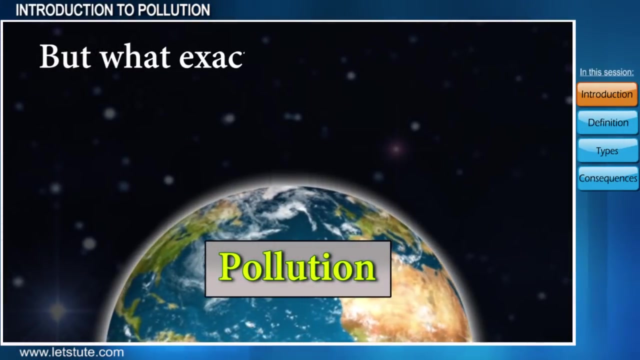 Hello everyone. Today we'll be looking into a very important topic, Something that affects everything on this planet, irrespective of where they are. We read everyday newspapers, magazines about it causing irreplaceable damage to earth, and it's increasing every passing year. Yes, it is the problem of environmental pollution, But what exactly is this pollution? 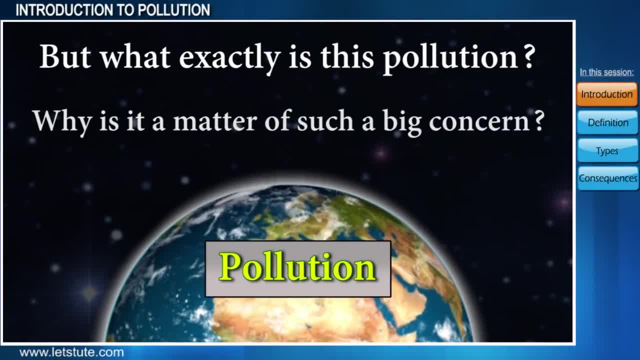 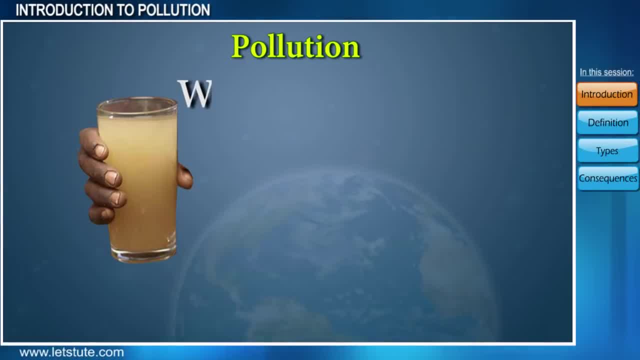 Why is it a matter of such a big concern? To understand that, just consider: I gave you this glass of water to drink. Will you drink it? And if I ask you the reason for that, you would say that it's not clean and hence undesirable or undesirable. 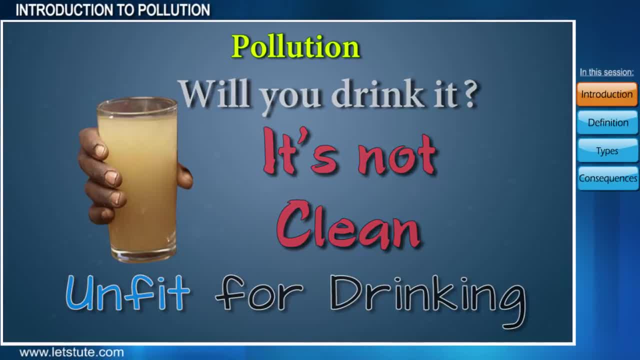 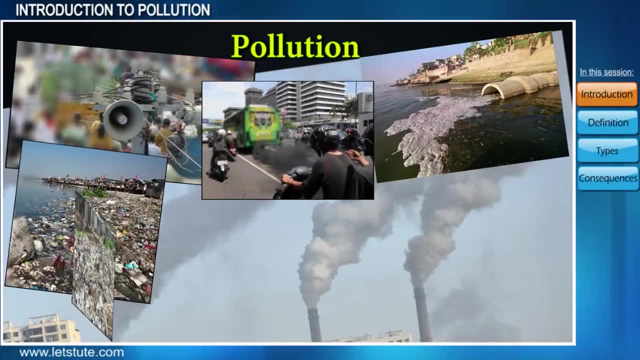 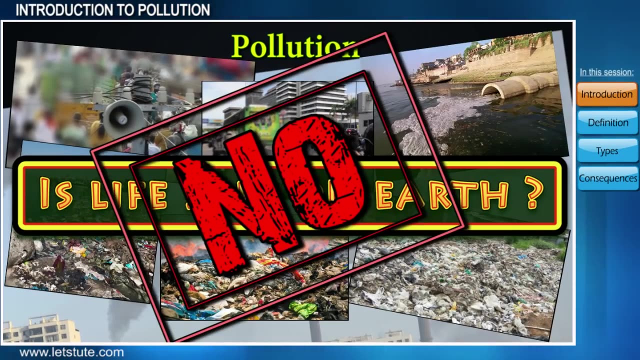 Unfit for drinking right Along the same lines, or just on a broader scale, consider our surrounding, where we keep on adding impurities on a daily basis. Will then be our environment safe for existence of life? No right. So to define pollution, we need to look into three aspects. 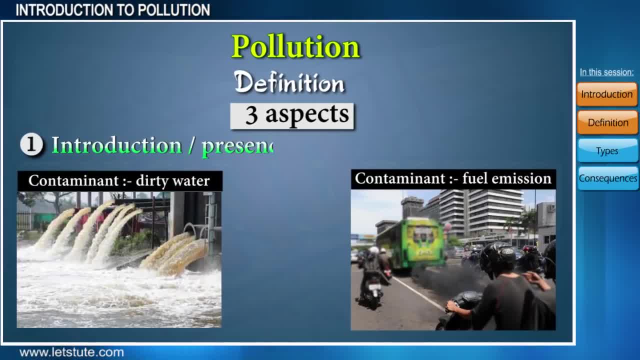 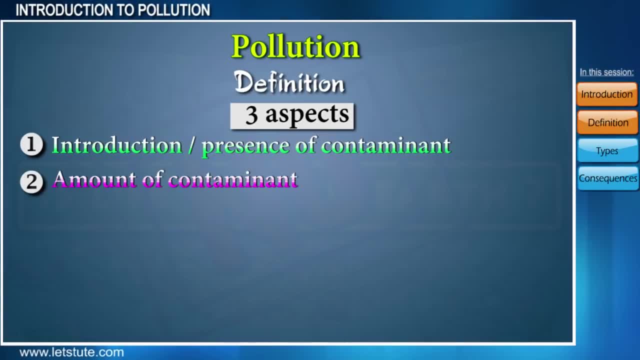 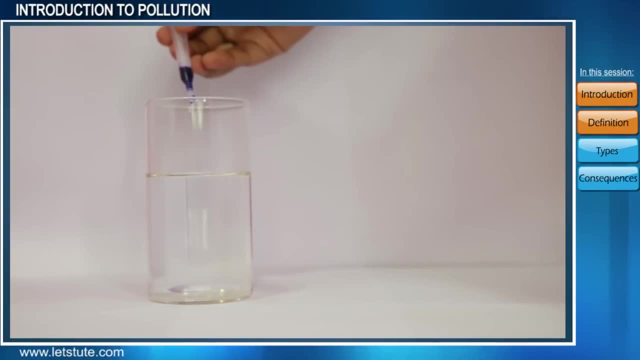 First, if the contaminant is being introduced or present in our surrounding. Secondly, the extent to which it is present. To understand this, let's consider a clean glass of water To which we add just one drop of ink, And to another glass of water we poured an entire. 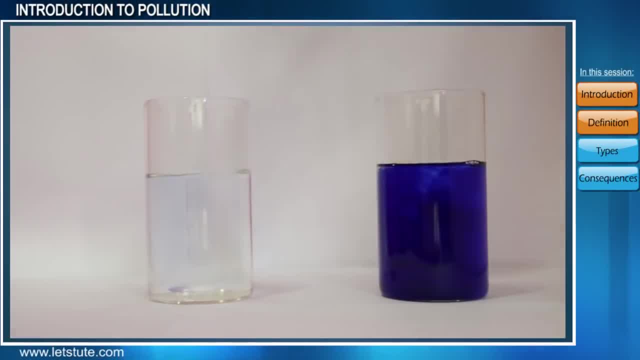 bottle of ink And we stir both the glasses of water, So which one will you call polluted? If we go to sea, both the glasses of water will be polluted, So which one will you call polluted? Let's see what happens if we add two drops of ink to the second glass of water. 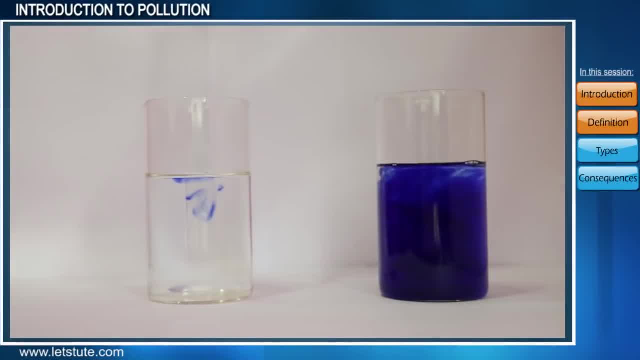 So which one will you call polluted And how will we know which one is the contaminant? In this example, both the glasses of water have contaminant, which is the ink which we added In the first case. the drop of ink just disperse in the water And the water 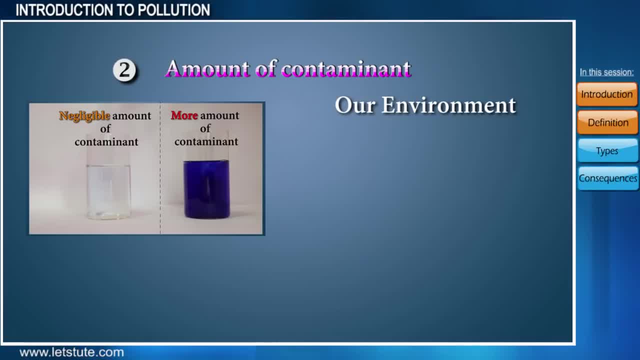 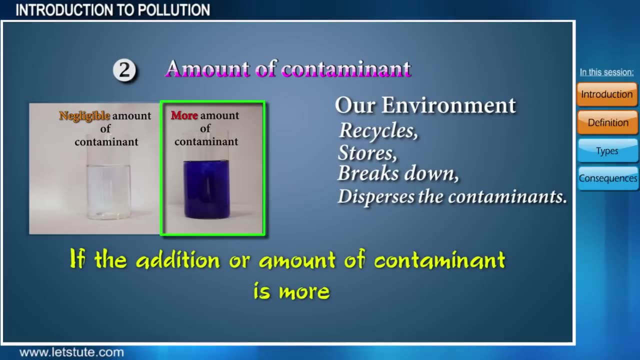 is almost clear, indicating negligible amount of contaminant. But the second glass has more contaminants, by recycling, storing, breaking it down or dispersing them. But if their addition is at a rate faster than what our earth can hold, only then we. 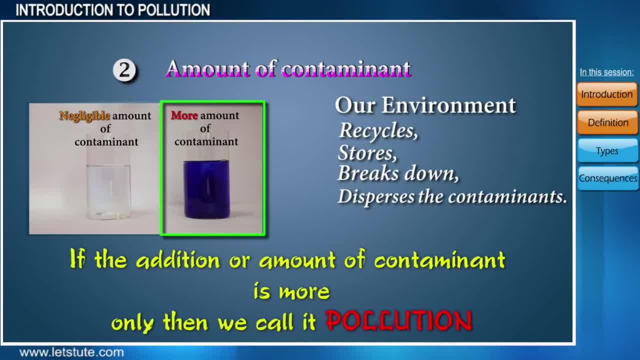 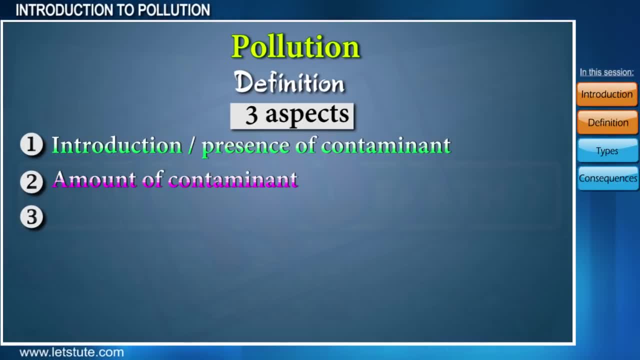 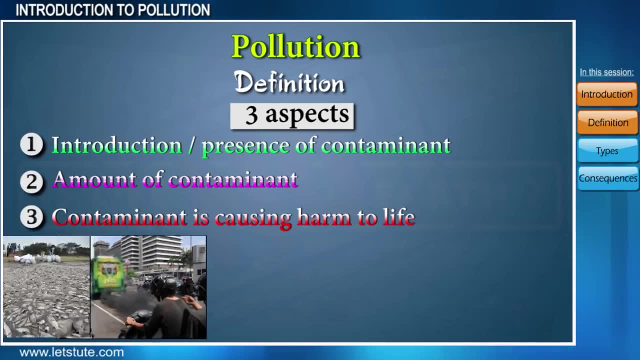 call it pollution. I hope you are understanding. Now we come to the third aspect, that is, whether the presence of contaminant is causing harm or discomfort to living beings or our environment as a whole. So, considering these three aspects, we can now define pollution as the introduction. 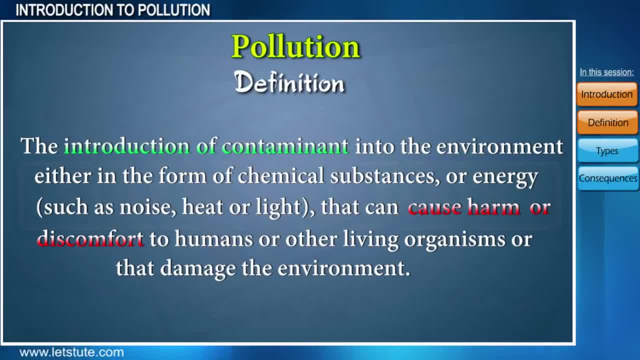 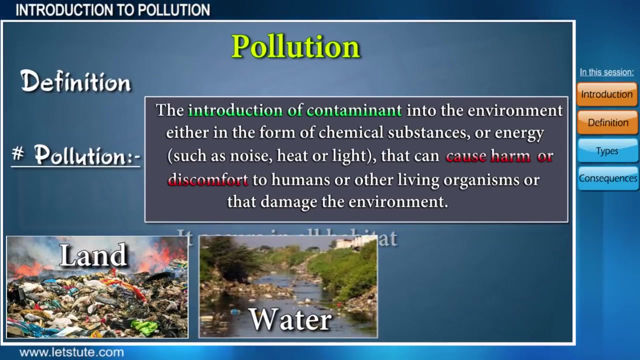 of contaminants into the environment, either in the form of chemical substance or energy that can cause harm or discomfort to humans or other living organisms that damage the environment. Pollution can occur in all habitats, may it be land, sea, fresh water or in the air. 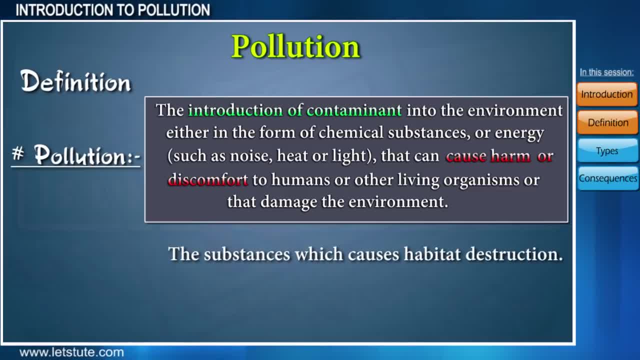 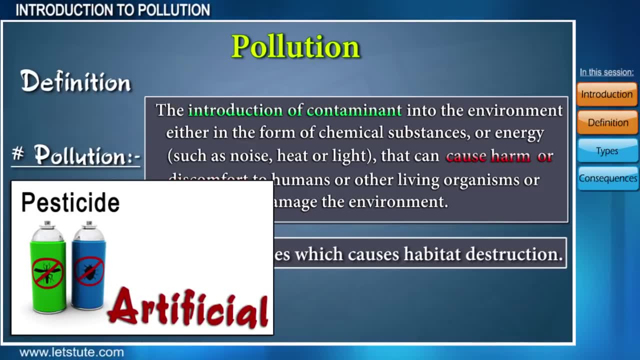 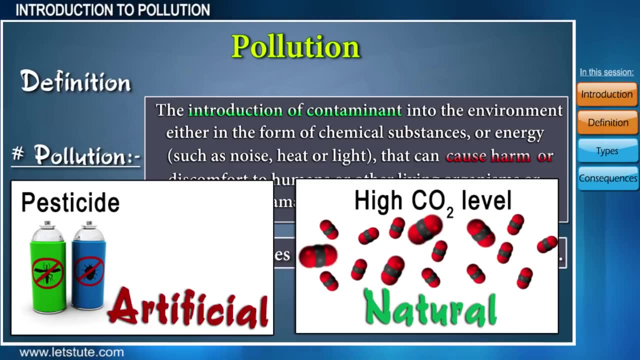 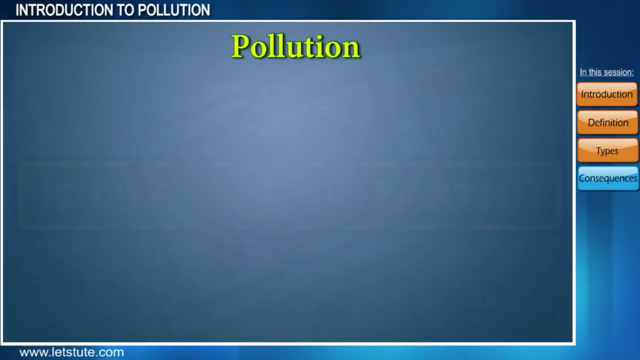 And the substances which causes this habitat destruction are called pollutants. They can be artificial or synthetic substances, such as pesticides, or naturally occurring substances, such as carbon dioxide, that occur in harmful concentration in a given environment, Based on the type of pollutant and the part of the environment which they affect there. 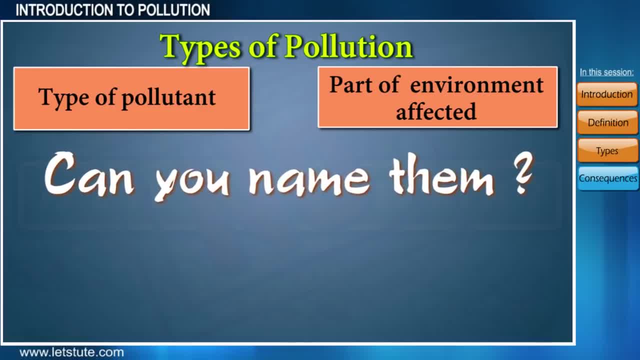 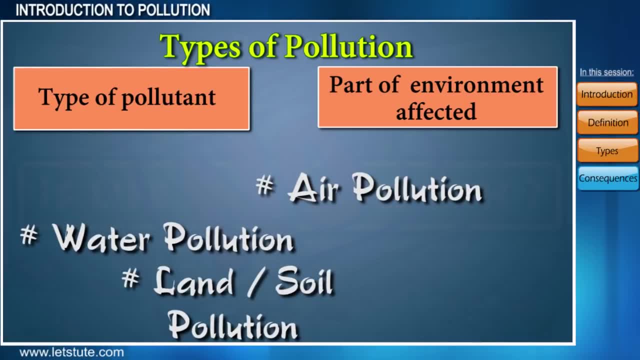 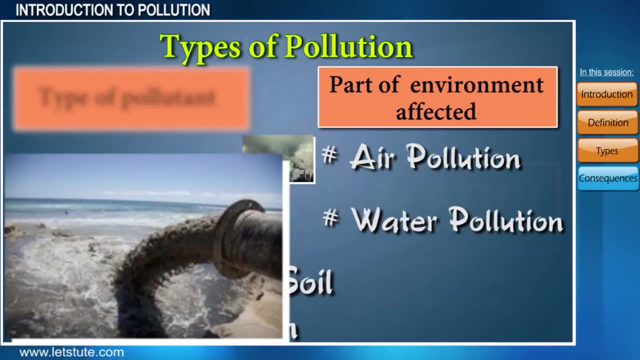 are different kinds of pollution. Well, if I ask you to name these types, most of us would say air, water, land or soil pollution. And here the three habitats, ie our atmosphere, water and land environment is getting affected, or we can say there is a decline in the quality. 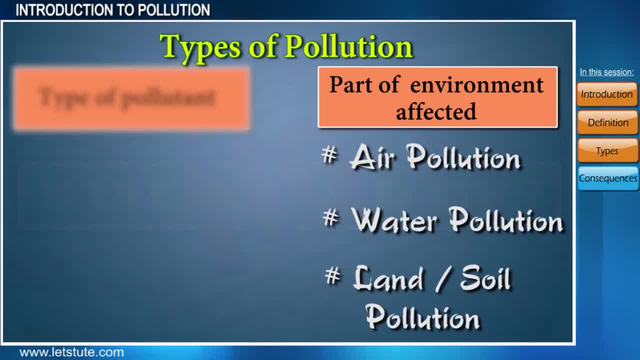 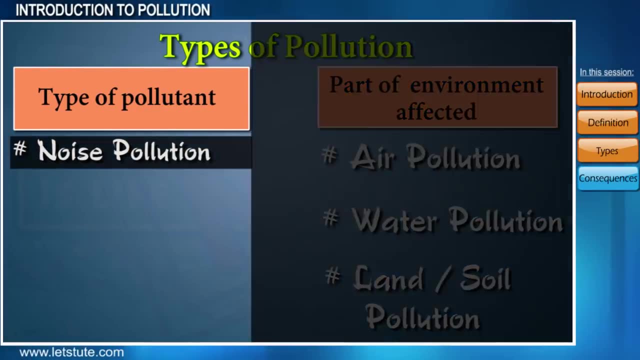 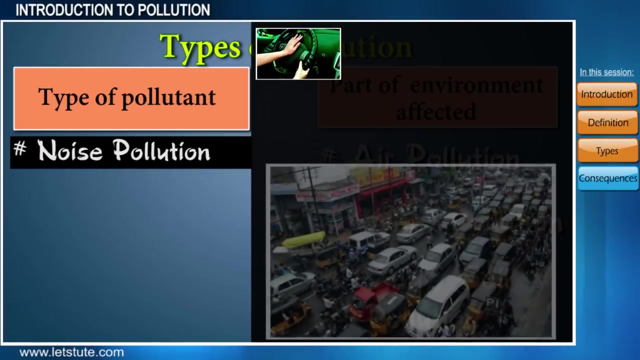 of these three components. but, friends, do you know there are some other kinds of pollution as well, the ones that depend on the type of pollutant or contaminant that is added. can you think of what they are? nice pollution, the sound generated from various vehicles during transportation, the honking of horns at traffic signals, the sound of loudspeakers. 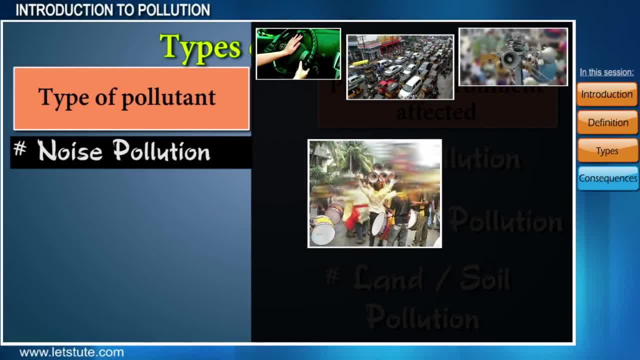 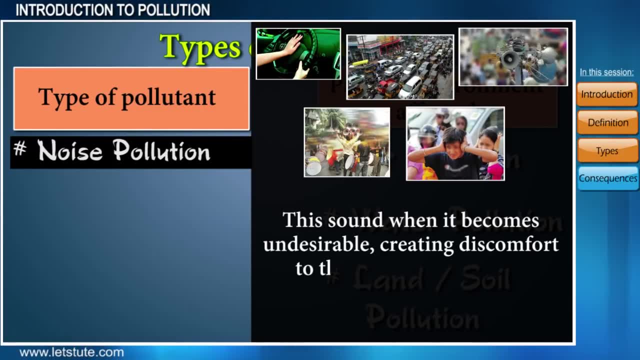 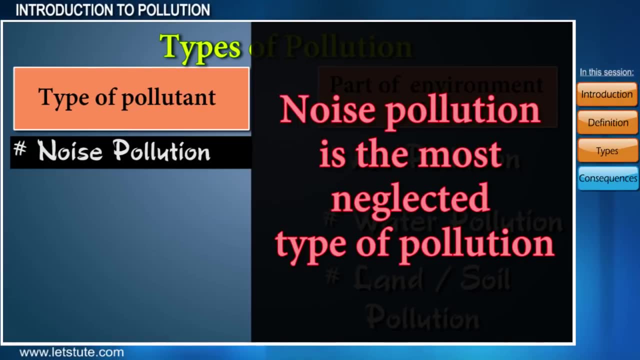 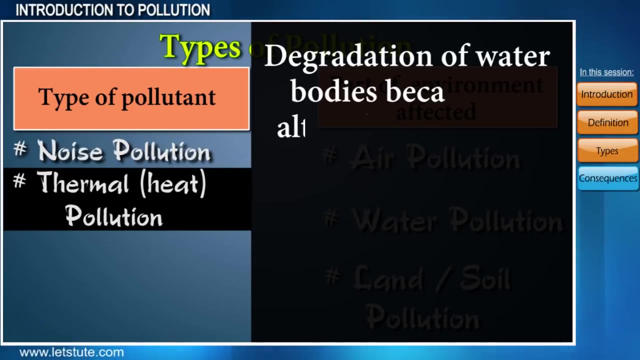 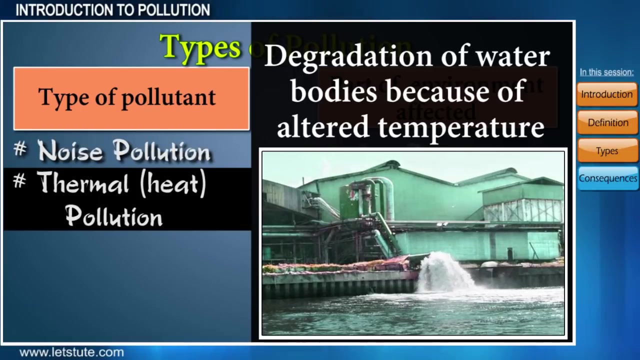 playing drums, etc. at times become annoying. right this sound when it becomes undesirable, creating discomfort to the years. we call it noise pollution. thermal pollution occurs when water bodies are degraded in terms of altering their temperatures. this especially occurs in thermal and nuclear power plants where large amount of water is. 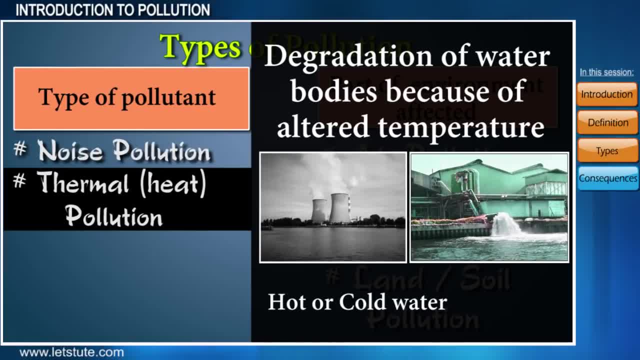 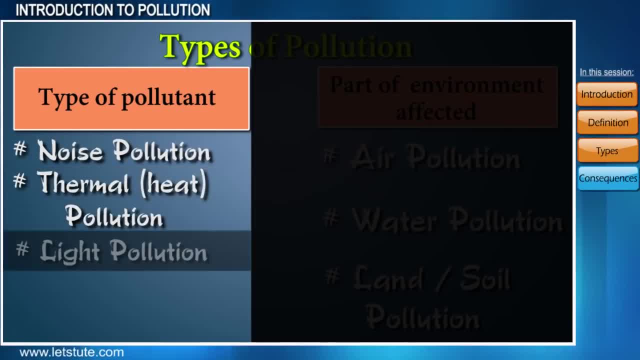 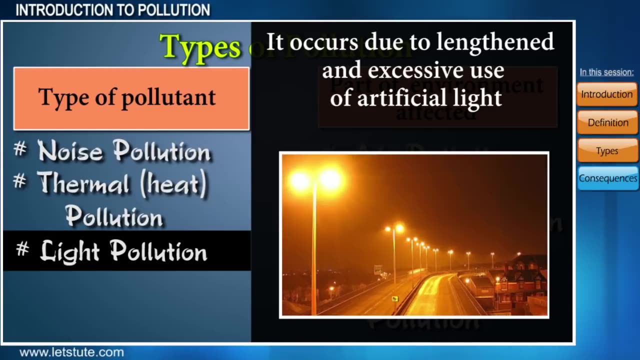 used for heating and cooling purposes and they are released into natural water bodies. light pollution- light pollution, you might be wondering. how can light be a form of pollution, right? light pollution occurs due to lengthened and excessive use of artificial light, such that it results in brightening. 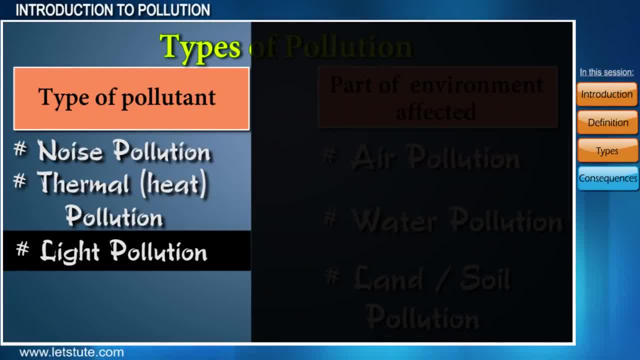 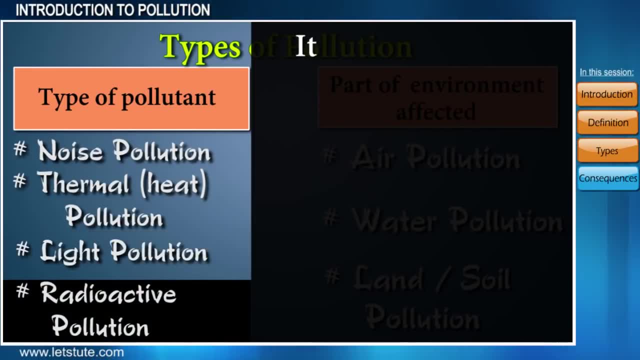 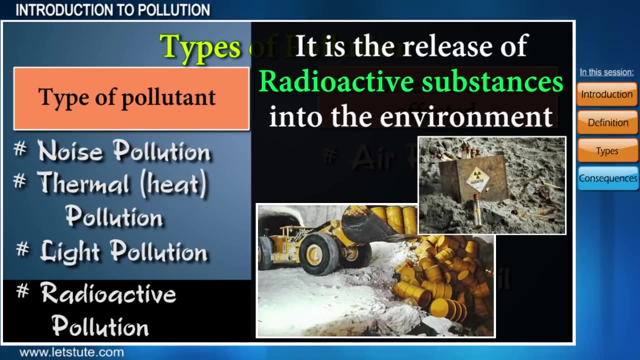 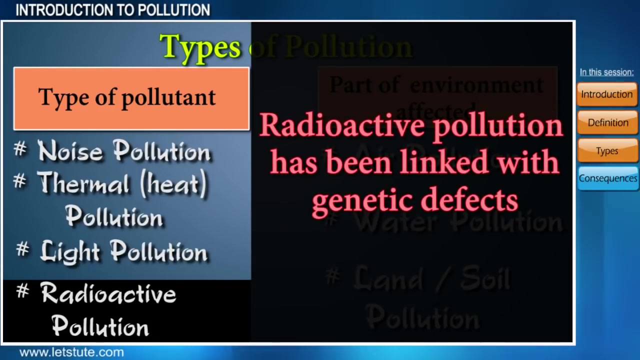 of the skies at night. radioactive pollution, like any other kind of pollution, it is the release of something unwanted into the environment, that is not suitable for the environment, and it is the other environment. these processes can be used to create a natural environment. in this case, the unwanted thing is radioactive material. 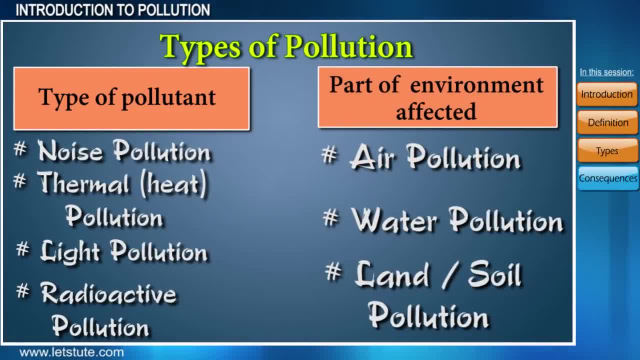 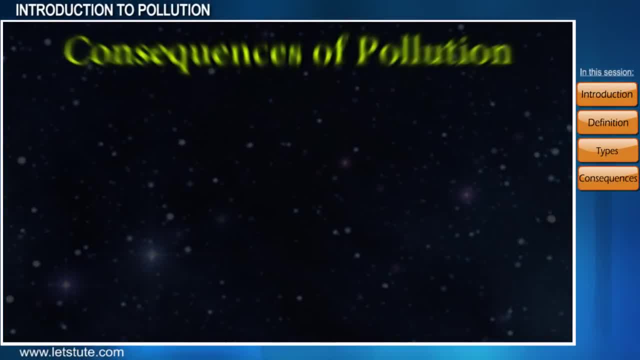 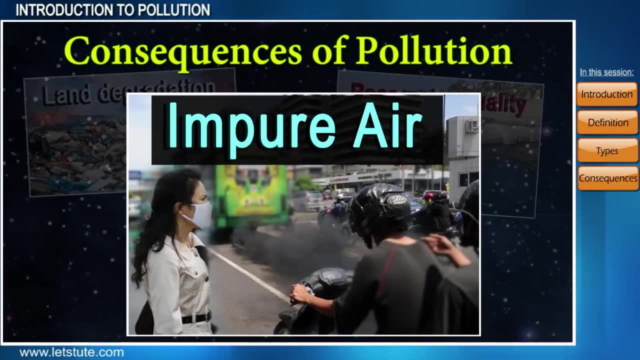 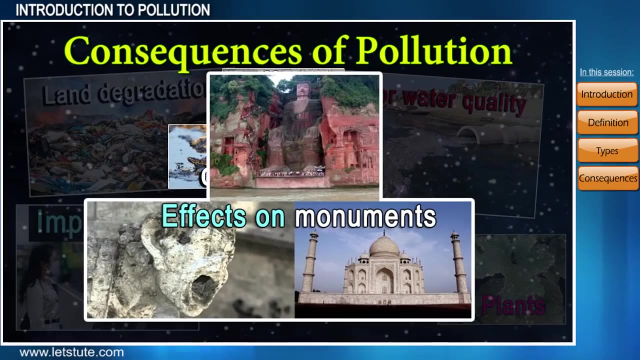 friends, don't worry, we will be studying the individual types of pollution in detail in our upcoming sessions, and one thing we must note here is that each type of pollutants may come from different sources and may have different consequences, but the ultimate truth result of all these is environmental degradation. They all have harmful effects on life and 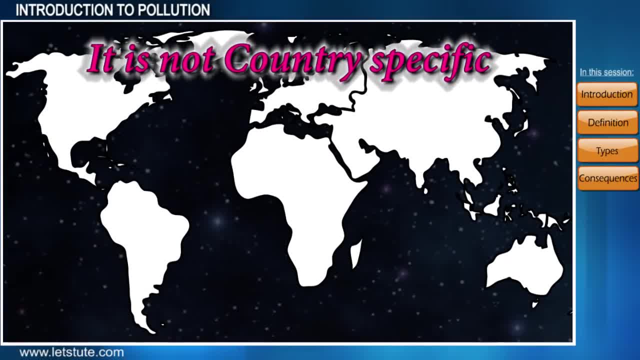 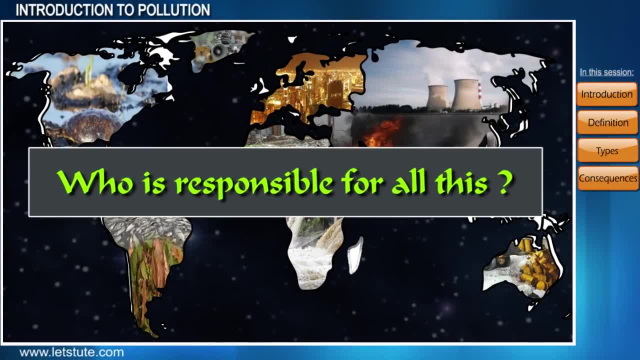 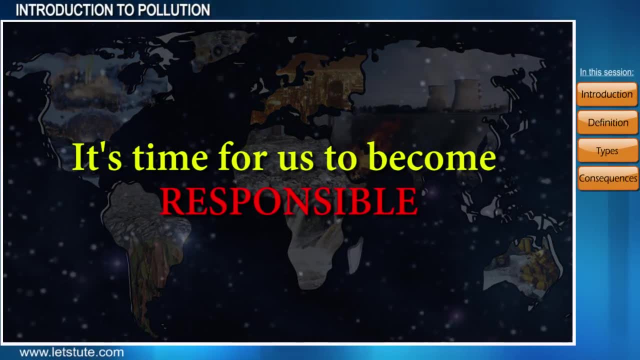 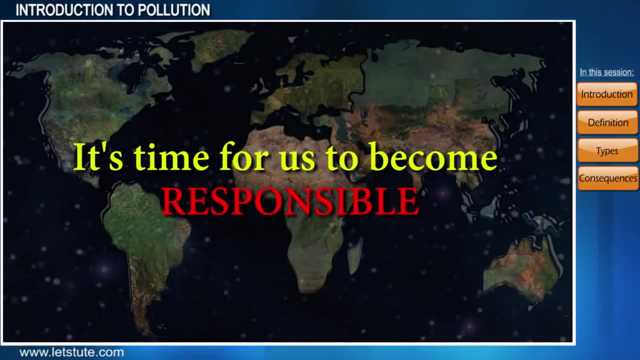 environment. These issues are not country specific, but it affects the entire planet and it is all happening because of us humans or the activities done by humans. So it is our responsibility to become environmentally cautious individuals. We all must be aware of our deeds. We must ensure our activities should cause minimum damage to our environment. 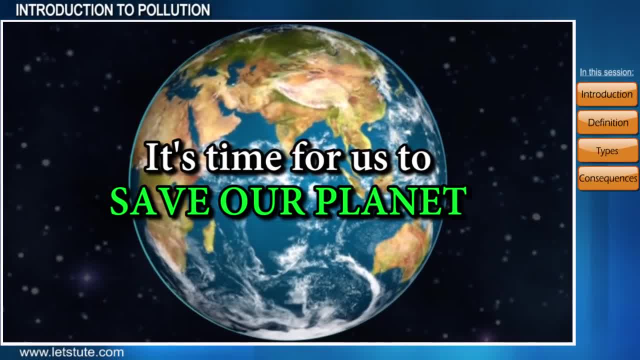 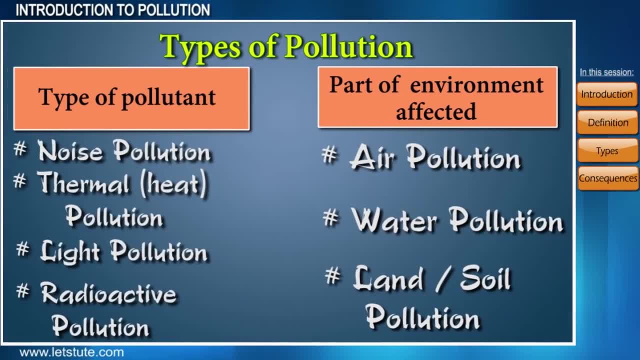 Only then we can ensure sustainable development. So that's it for today. For our further sessions on environmental pollution, please stay tuned with us. If you like this session, give us a thumbs up and don't forget to subscribe to our channel. 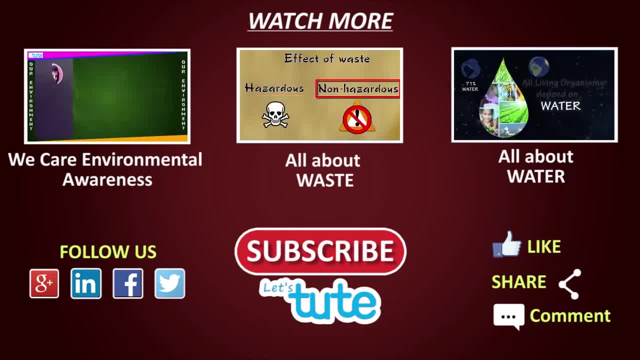 Till we meet the next time, keep watching, keep learning. Thank you.